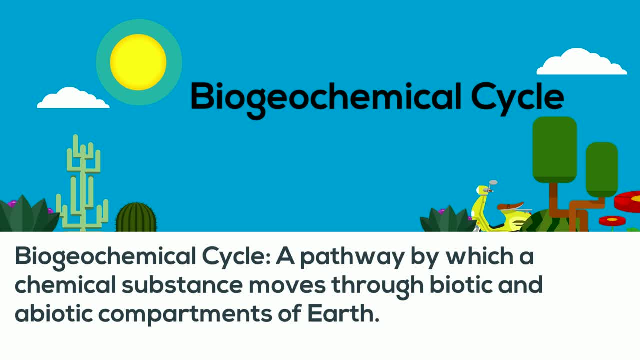 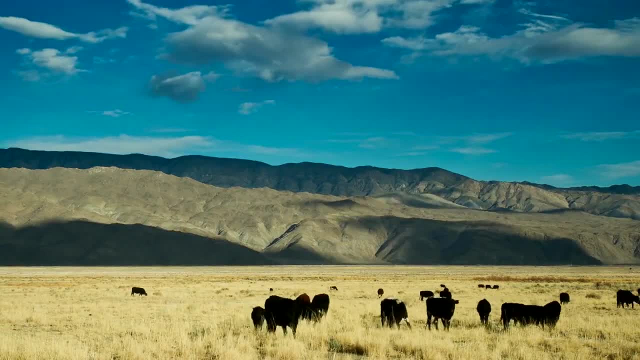 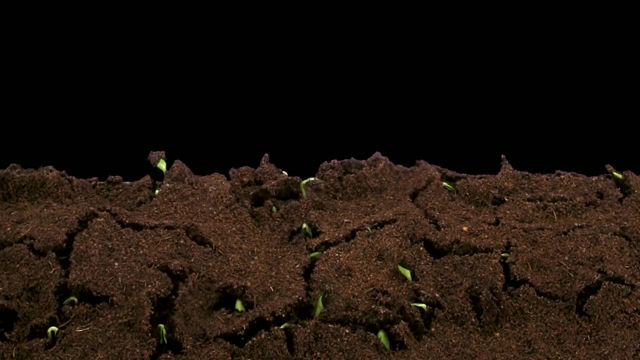 a chemical substance, moves through a biotic and the abiotic compartments of earth. Although phosphorus is not found in the atmosphere, it still plays a very important role in plants and animals on earth. Phosphorus is essential for plant and animal growth, as well as the 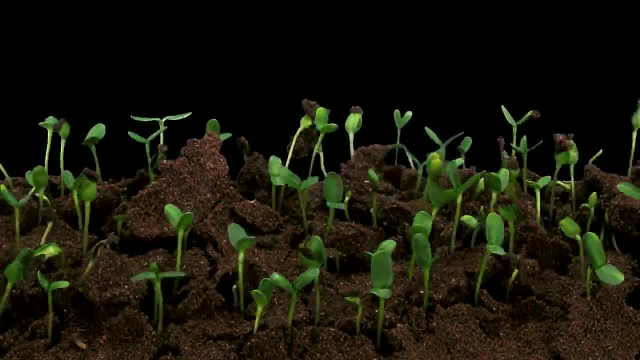 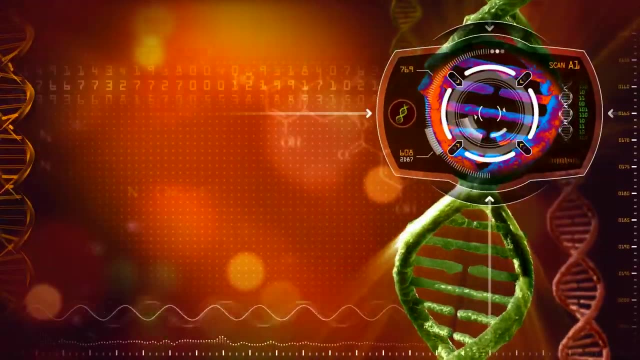 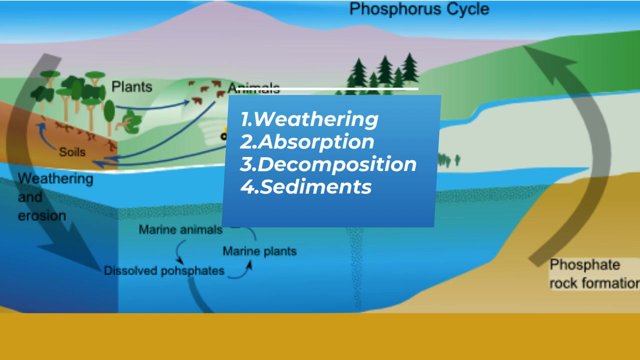 health of microbes inhabiting the soil. Phosphorus is very important for the production of DNA and RNA, helps to make up cell membrane and the production of ATP. The phosphorus cycle is a slow process and involves four key steps: Step 1.. 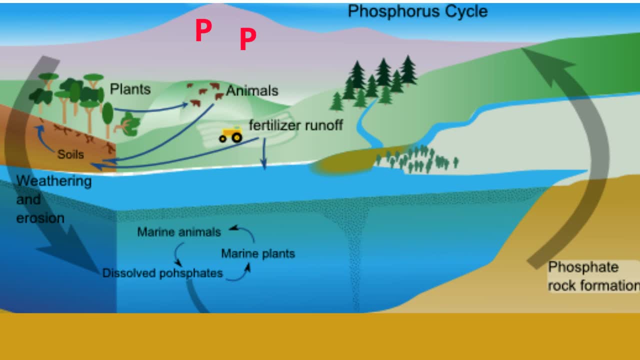 Step 1. Weathering: Phosphorus is found in rocks. Weathering, along with rain, breaks down the phosphorus in rocks and it travels to the soil and into water sources. Step 2 is absorption by plants and animals. Once in the soil, plants, fungi, microorganisms. 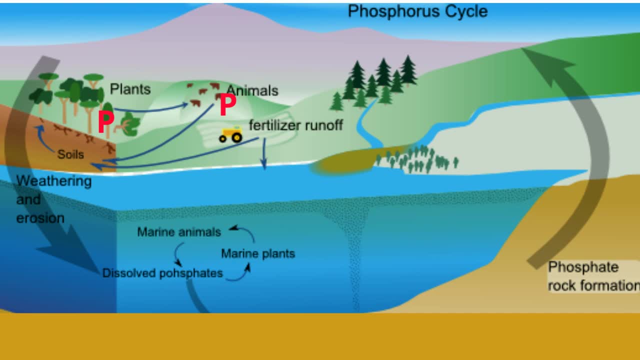 are able to absorb phosphorus and then grow. Some of it also makes its way to the ocean and fresh water, and animals are able to do that. Step 3. Phosphorus is absorbed by plants and animals Once in the soil. plants, fungi, microorganisms. 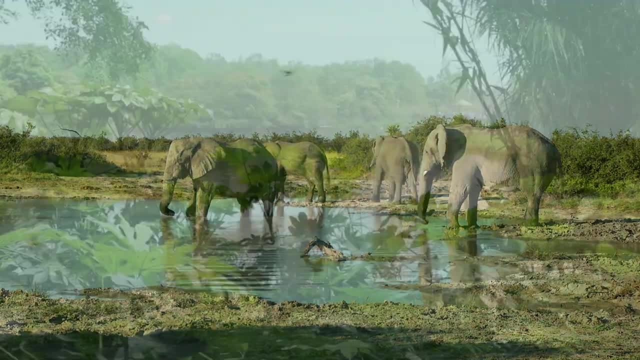 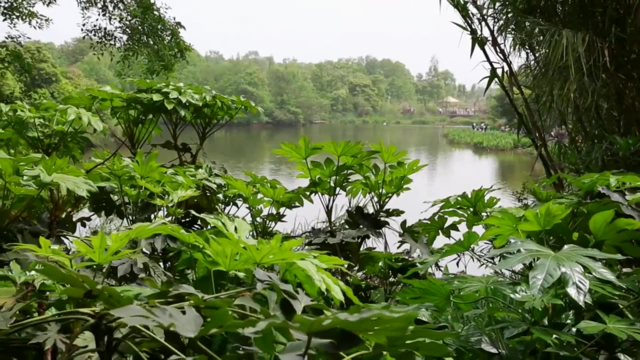 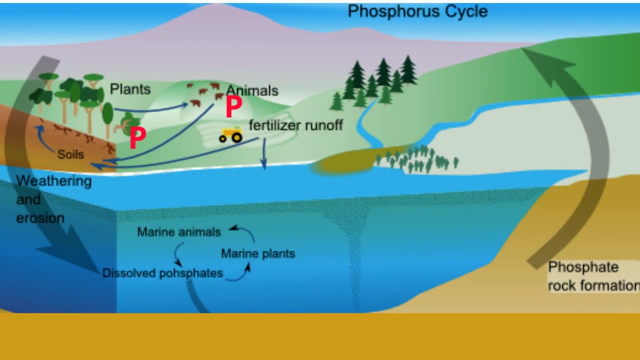 are able to drink this water and absorb the phosphorus. Plants absorb the water along with the phosphorus, and then the animals eat the plants and the phosphorus moves into the animal in this way also. Step 3. Step 3. Return to the environment by decomposition. Animals excrete waste and decomposers are. 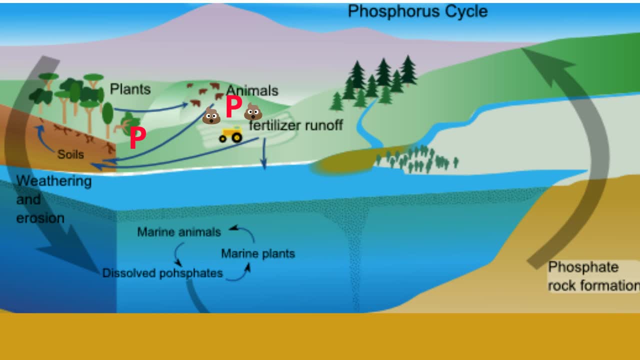 able to use the phosphorus in the waste material. Furthermore, when the plants and animals die, the bacteria convert the phosphorus into the waste material. This is called decomposition, Step 4. Settlement to rocks. Some of the phosphorus gets buried in settlement, which 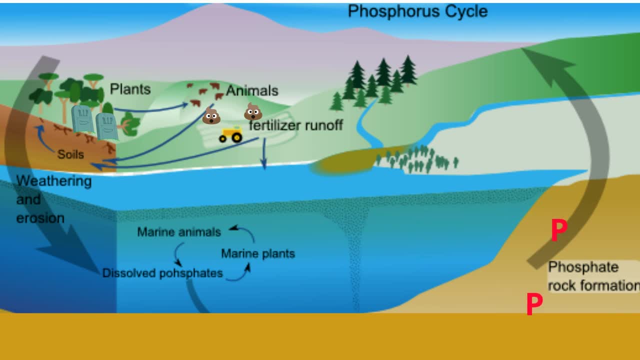 over time becomes rocks, and the cycle continues. Some of the phosphorus in the soil gets washed into the ocean, where a similar process takes place. Plants and animals in the ocean absorb the phosphorus, die and decompose, and some of the phosphorus ends up as the waste material. 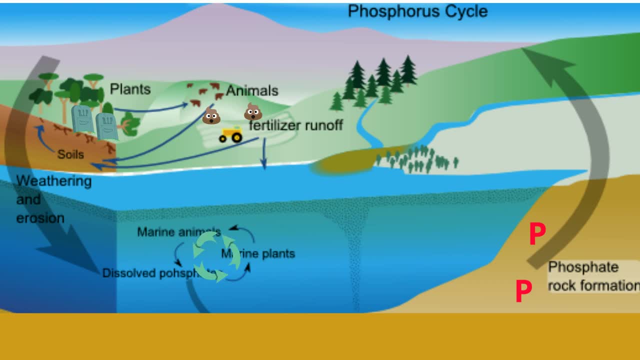 The phosphorus is then separated out of the water and is then transported to rocks and water sources. Step 5. The sediment is buried into the rocks. Some of the phosphorus gets sediments in the rock. humans have had a significant impact on the phosphorus cycle. fertilizers: